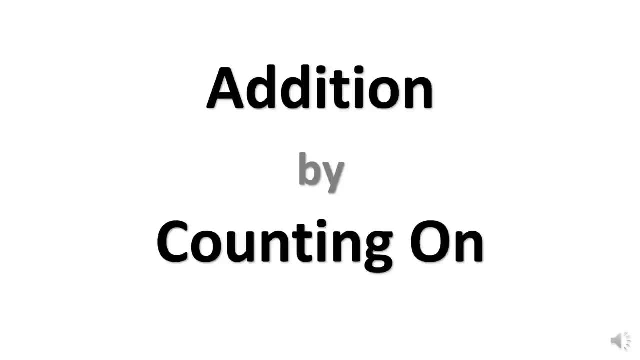 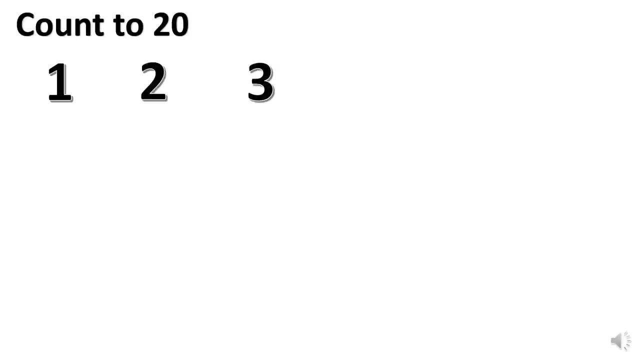 Hi everyone. today we are going to learn addition by using a very easy method called counting on, But first we need to recall back counting to 20.. Let's do it together: 12,, 13,, 14,, 15,, 16,, 17,, 18,, 19,, 20. 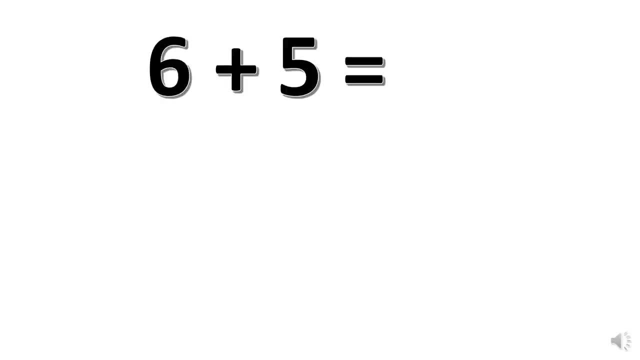 The first equation that we are going to do is 6 plus 5.. Which one is the bigger number here? 6, So we are going to start counting from 6.. Which one is the smaller number? Which one is the bigger number here? 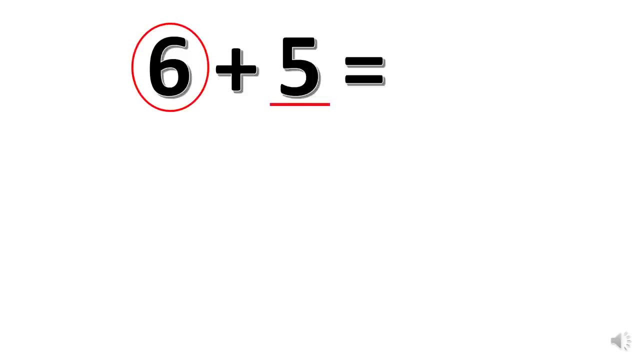 5. So let's have 5 fingers up everyone Now, starting from 6, let's count up 6, 7, 8,, 9,, 10, 11, So 6 plus 5 is 11. Here we have 8 plus 4.. 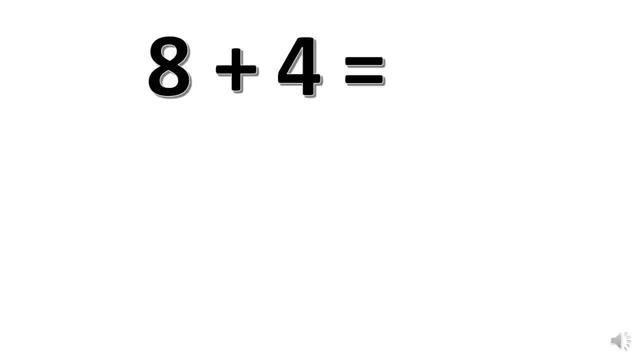 Which one is the bigger number here? 8. So we are going to start counting from 8.. Which one is the smaller number here? 4. So let's all have 4 fingers up Now, starting from 8, let's count up. 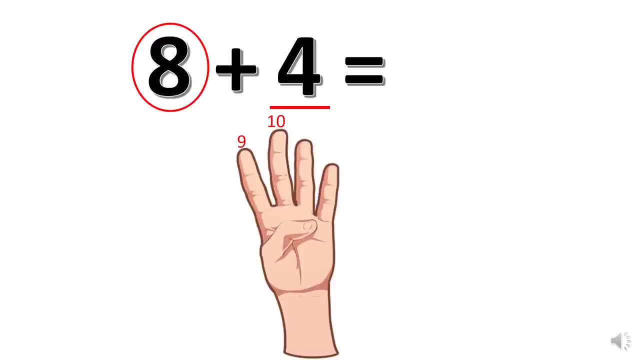 8,, 9,, 10,, 11,, 12. So 8 plus 4 is 12.. Now what about 9 plus 7?? Which one is the bigger number here? 9, So we are going to start counting from 9.. 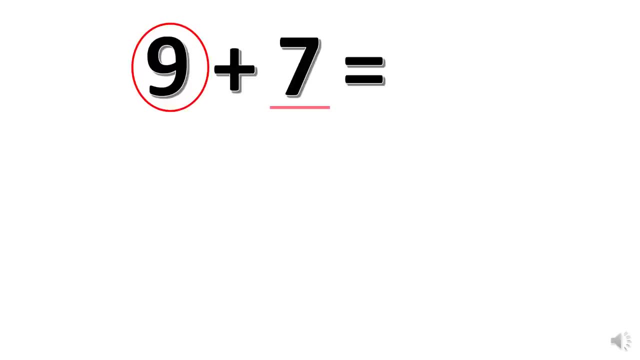 Which one is the smaller number here? 7 Now can you put 7 fingers up? Now let's start counting from 9.. We count up 9, 10, 11, 12, 13, 14, 15, 16, So 9 plus 7 is. 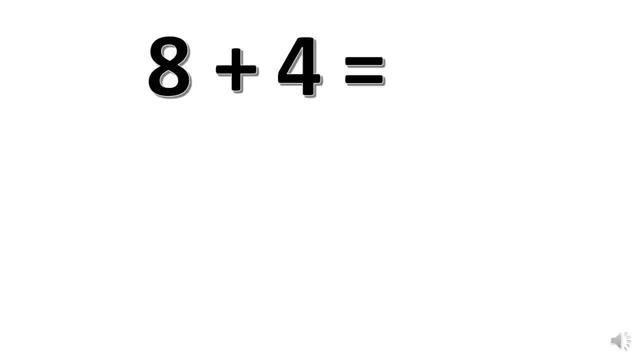 Which one is the bigger number here? 8. So we are going to start counting from 8.. Which one is the smaller number here? 4. So let's all have 4 fingers up Now, starting from 8, let's count up. 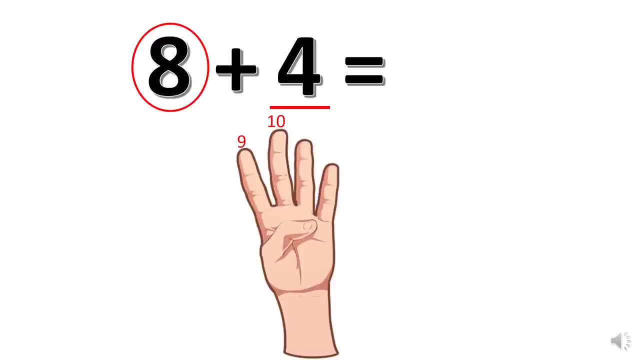 8,, 9,, 10,, 11,, 12. So 8 plus 4 is 12.. Now what about 9 plus 7?? Which one is the bigger number here? 9, So we are going to start counting from 9.. 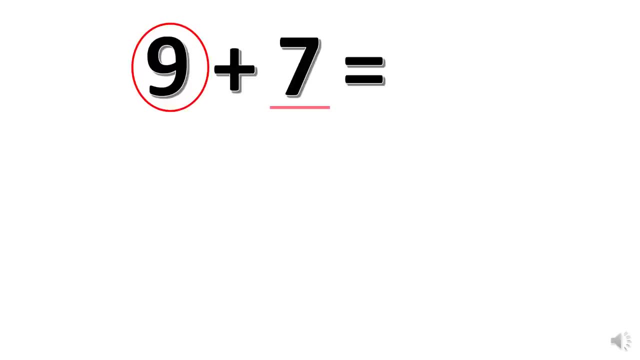 Which one is the smaller number here? 7 Now can you put 7 fingers up? Now let's start counting from 9.. We count up 9, 10, 11, 12, 13, 14, 15, 16, So 9 plus 7 is. 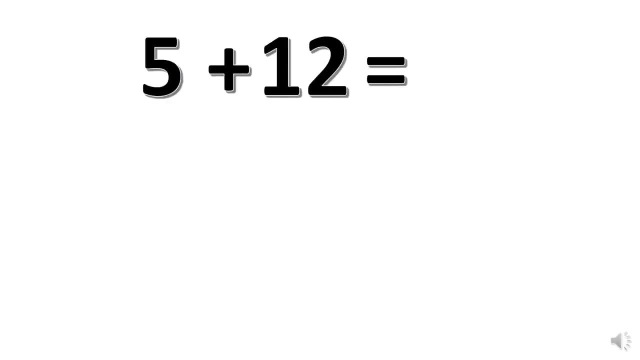 16. Next, what about 5 plus 12?? Which one is the bigger number here? 12. So we are going to start counting from 12.. Now, which one is the smaller number here? 5. So let's all have 5 fingers up. 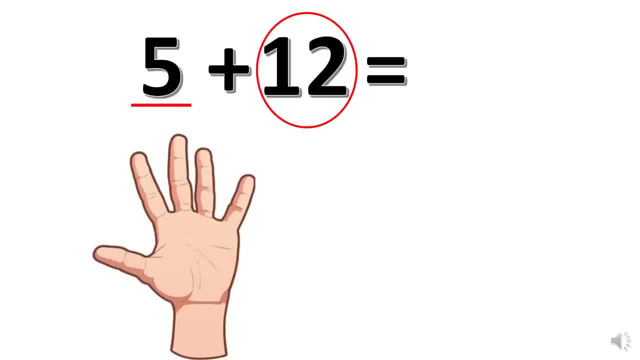 Good Now, starting from 12,. let's count up 12, 13, 14, 15, 16, 17. So 5 plus 12 is 17. We have 3 plus 16.. So we are going to start counting from 12.. 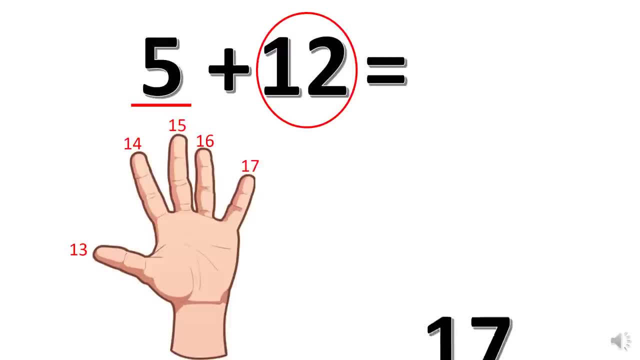 So 5 plus 12 is 17. So 5 plus 12 is 17. We have 3 plus 16. 15. So 5 plus 12 is Which one is the bigger number here? Sixteen. So we are going to start counting from sixteen. 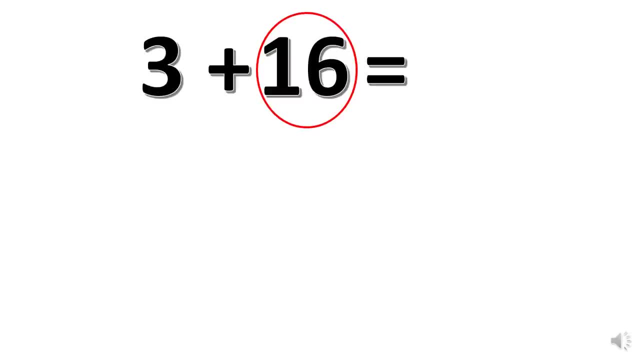 Which one is the smaller number here? Three, So let's all have three fingers up. Now we are going to start counting from sixteen. Let's count up Sixteen, Seventeen, Eighteen, Nineteen, So three plus sixteen is. 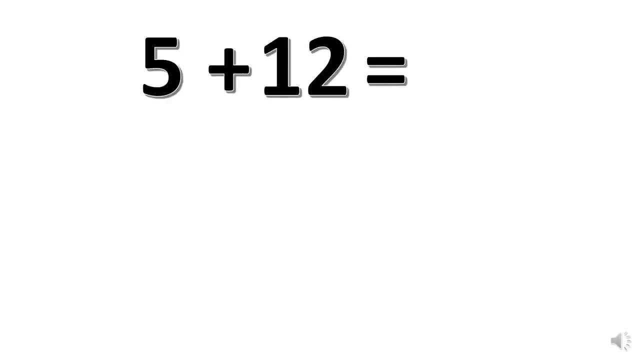 16. Next, what about 5 plus 12?? Which one is the bigger number here? 12. So we are going to start counting from 12.. Now, which one is the smaller number here? 5. So let's all have 5 fingers up. 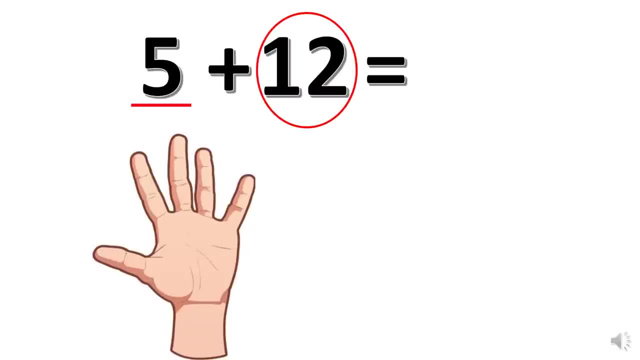 Good Now, starting from 12,. let's count up 12, 13, 14, 15, 16, 17, So 5 plus 12 is 17. We have 3 plus 16.. So 5 plus 12 is. 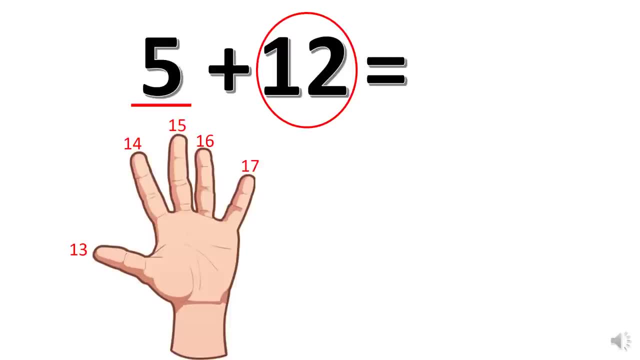 17. We have 3 plus 16.. So 5 plus 12 is 17. 17 We have 3 plus 16.. 16: Which one is the bigger number here? 16. So we are going to start counting from 16.. 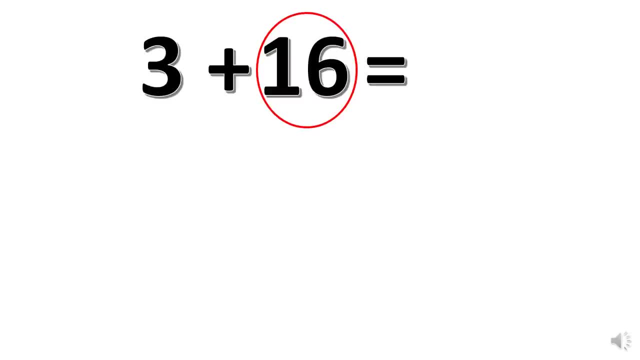 Which one is the smaller number here? 3, So let's all have 3 fingers up. Now we are going to start counting from 16.. Let's count up 16, 17, 18, 19, So 3 plus 16 is 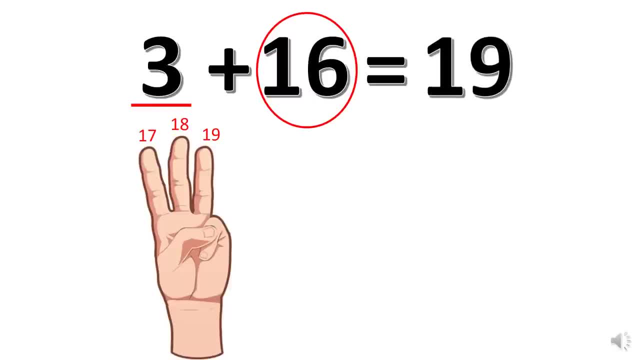 19. Next, what is 6 plus 7?? Which one is the bigger number? 6 or 7?? 7, So we are going to start counting from 7.. Now, which one is the smaller number here? 6, So let's have 6 fingers up. 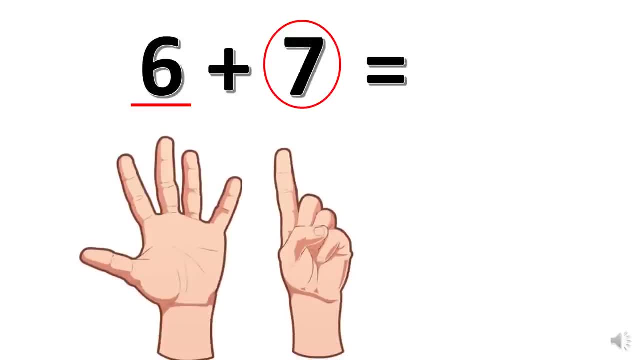 Now let's start counting from 7.. Let's count up 7, 8, 9, 10, 11, 12, 13, So 6 plus 7 is 13. That is all from me today. I hope you enjoyed the lesson. 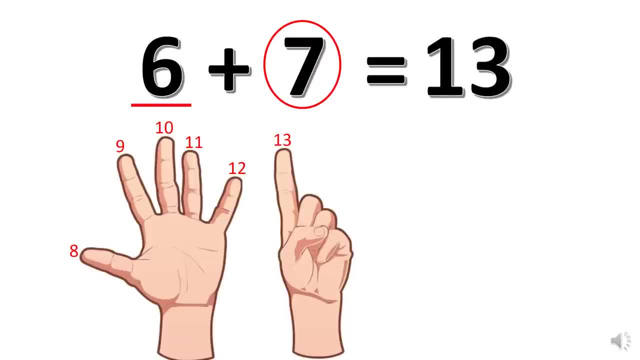 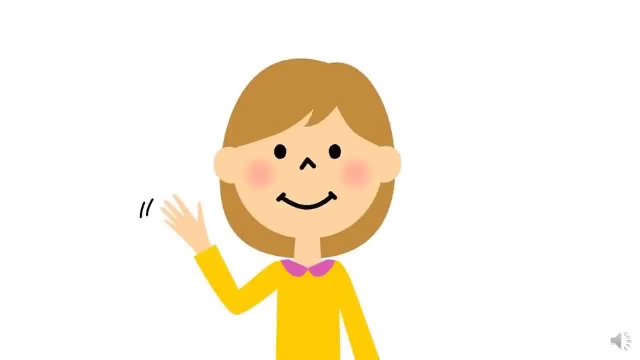